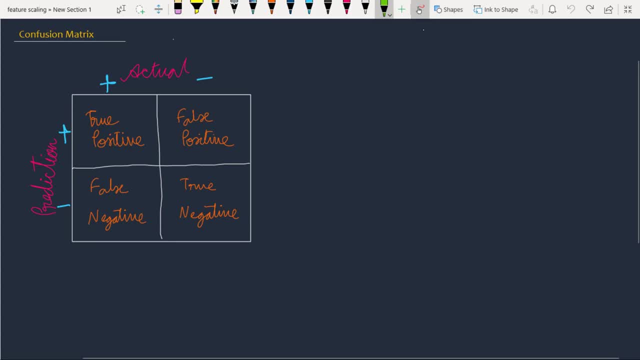 it is the easiest to understand the confusion matrix of: okay, so suppose I am working on a binary classification where Y represents the ground truths and Y represents the Y-hat represents predictions. okay, so how many possible cases may arise? suppose a ground truth, they take the value 0 and 1. so it is obvious that Y pred will not be equal to ground truths always. 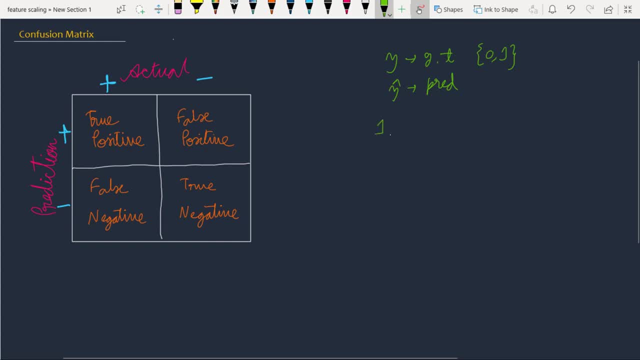 so it may happen that ground truth is 1 and Y-hat is also on. it may also happen the ground truth is 0 and the Y-hat is 0.. so these two cases you can see that our Y-hat coincides with the ground truth. so that means 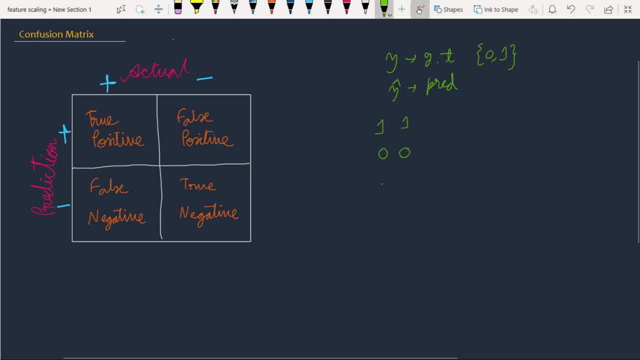 these two are correct predictions, but it may also happen that ground truth is 0 and Y pred is 1 and in. in the last case, it may happen that the ground truth is 1 and Y pred is 0. so you can see that these two are correct predictions, but these two are wrong predictions, okay. so 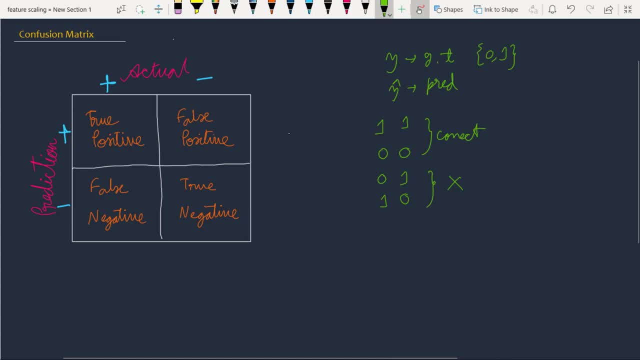 now a confusion matrix basically encodes this information over all the data points. okay, so confusion matrix basically contains all the data points that lies in the cross validation set and it encodes this information: how many it got correct and how many it got uncorrect. so let 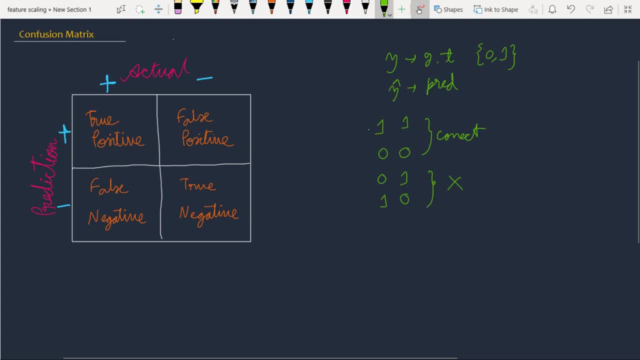 us classify these four cases. well, in this first case, you can see that the ground truth is positive as positive and zero as negative, which is the convention. so in the first case i have, ground truth is positive and our model also produces a positive result. so it is a case of true, positive. 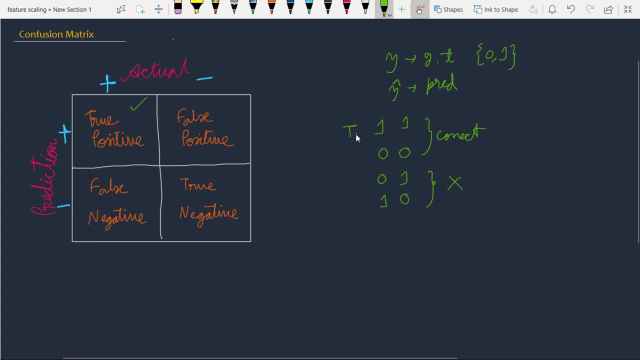 this is we call as true positive. in the second case you can see that ground truth is negative and the prediction is also negative. so it is a case of true negative. so we call it true, negative. but in this case you can see that the ground truth is negative but our model has predicted. 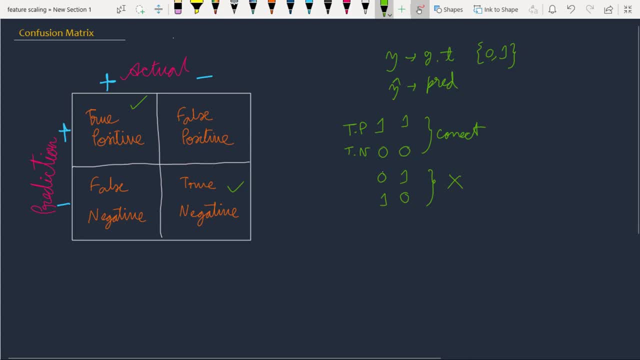 that it is a positive case, so it means that it is a false positive. it is a false positive. this is the false positive one, and in this last case, you can see that the ground truth is positive, but our model has predicted a negative, so this is false negative. this is the. 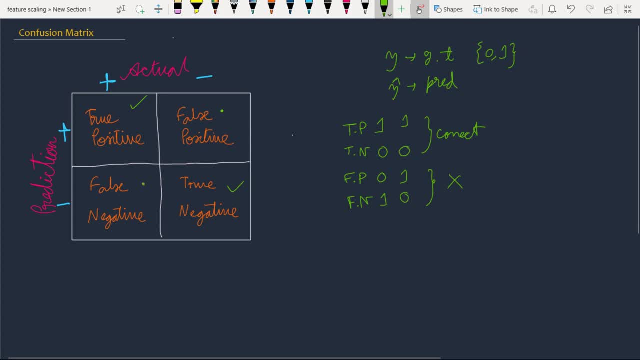 case corresponding to false negative. so a confusion matrix contains all these informations and the informations are about the cross validation set. okay, I hope the concept of confusion matrix is pretty much clear now. now we are going to see what is the definition of accuracy, so let me write down the 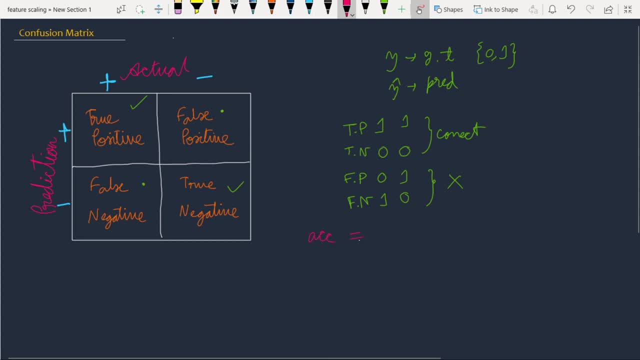 formula of accuracy. accuracy is basically equal to number of correct predictions divided by total. so what does a total means? total means the summation of true positive, true negative, false positive and false positive, negative, and the correct predictions are only the summation of true, positive and true negative. so I can actually write down the formula here: true positive plus. 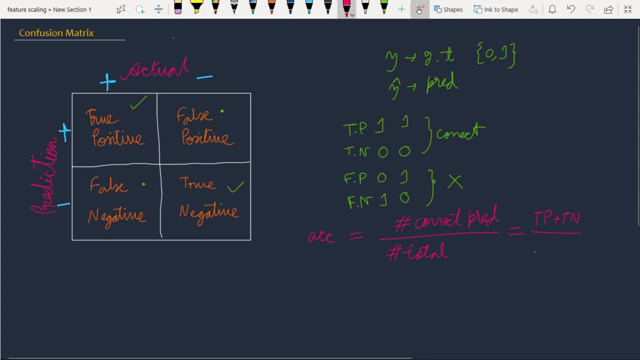 true negative divided by true positive plus true negative plus false positive plus false negative. so this basically means how many it got correct over the all the dataset. now we are going to find another parameter, which is known as F1 score. but before F1 score, I need to tell you two other definitions: the 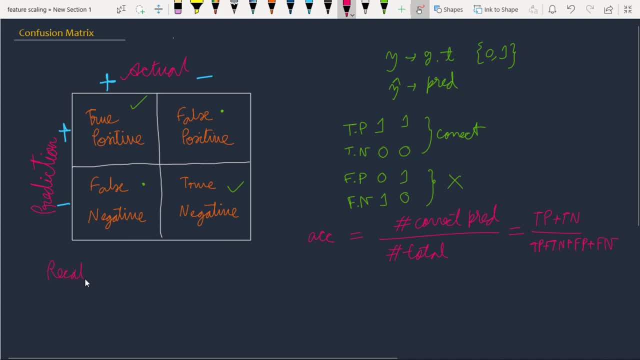 first one is recall. so what is a recall? so recall, basically, is the ratio of true positive to the summation of true positive and false negative. so the formula looks something like this: true positive divided by true positive plus false negative. and we have an other formula here which is: 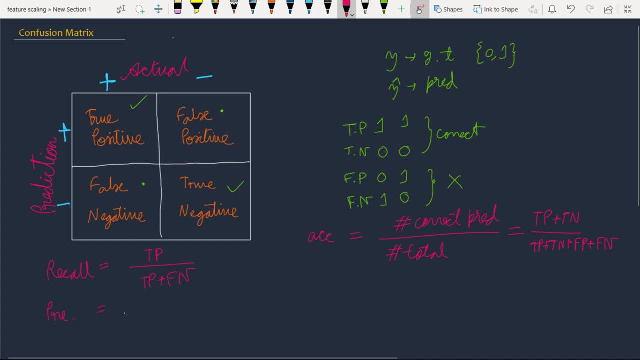 known as precision, which is given by the formula of ratio of true positive to the summation of true positive and false positive. so in the numerator we will have true positive and in the denominator we will have true positive plus false positive. now, the main thing that we 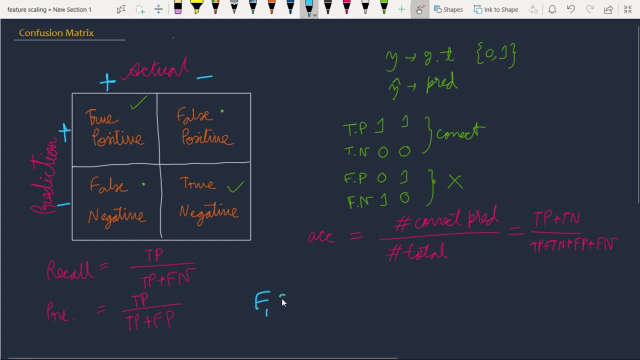 were looking for, which is f1 score, which is equal to the harmonic mean of recall and precision. well, if you don't know what a harmonic mean is, then don't worry, it is just referred to as this one: two times recall, times precision divided by recall plus precision. and to remember the formula of recall, you just 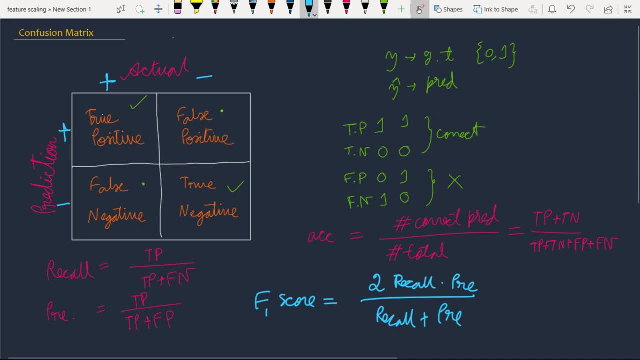 take this the first column, okay, and to remember the formula of precision, just take the first row and remember the true negative. we don't consider this true negative in our formula of f1 score. so i hope that you have learned this formula and if you have any questions, please do not. 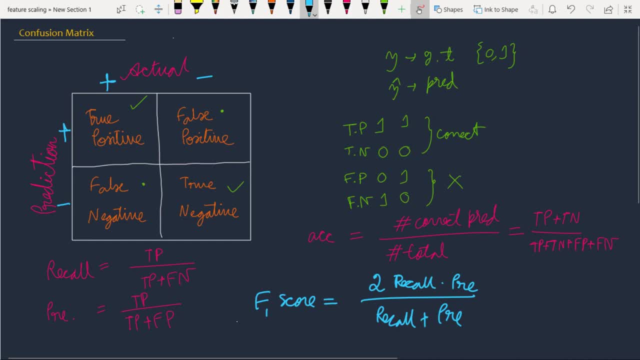 hesitate to ask. in the comment section below- and i hope that this one- this was pretty clear and i am again mentioning that we use the confusion matrix to derive all these parameters, that is, accuracy, scores, f1 score and recall and precision. now let me tell you, uh, why we need this kind of things. 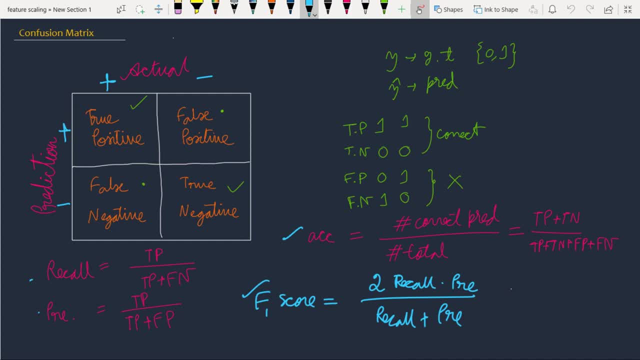 well, we need this kind of formulae to just examine how good our model is, because obviously we need some uh values to see if our model really works or not. so let's go ahead and look at our model and see if our model really works or not. so let's go ahead and look at our model and see if our model 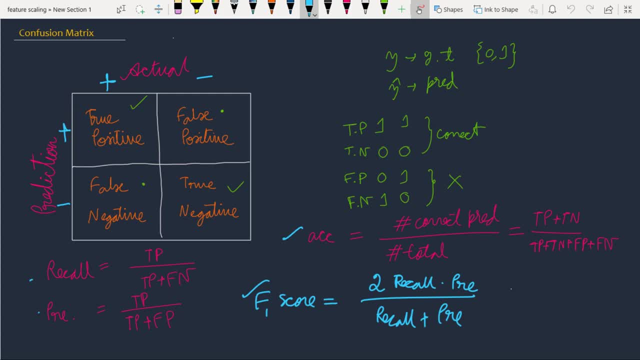 well or bad on a data set. so, uh, the f1 score and accuracy score are the values that we check to determine whether our model is a good model or a bad model. so that was all for this conceptual portion, and now i am going to show you how you can derive these values using our favorite library. 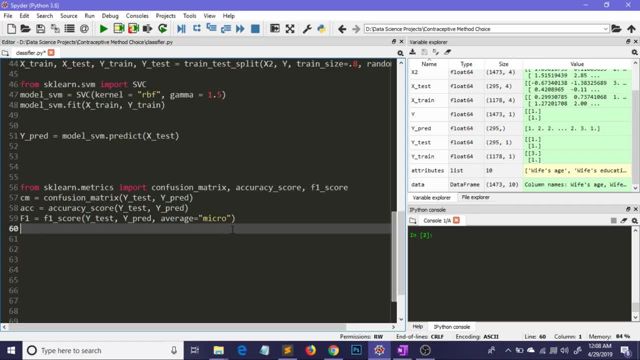 which is scikit-learn. to demonstrate the concept of confusion, matrix, accuracy score and f1 score in scikit-learn, i have taken an example of multi-class classification. well, intentionally i have taken a multi-class classification instead of a binary classification, because i wanted to show you that we can easily extend our concept of confusion, matrix and 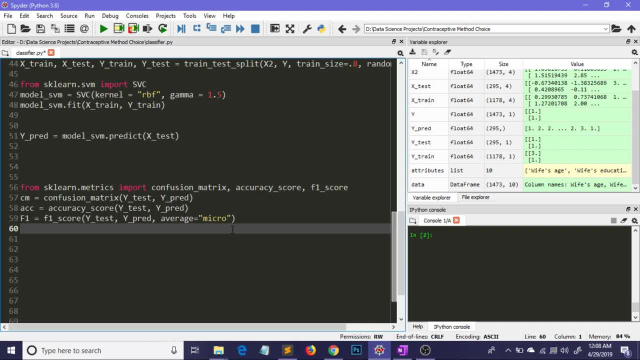 f1 score and accuracy score beyond just two classes. okay, so this is a tri-class classification. that means we have three classes to classify the data points. so i have done the classification model already, so you don't need to actually worry about this code in the model section. 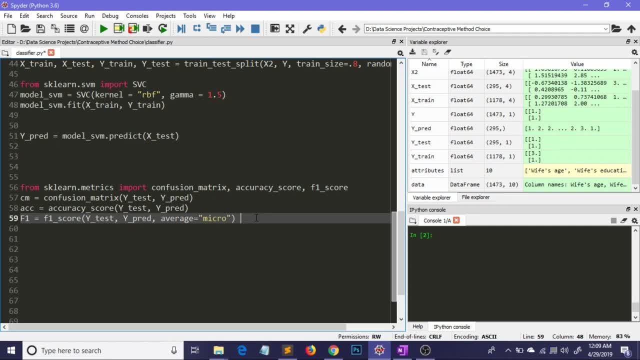 because this will work for any classification problem. so what we need to do? first we have to import some classes from a module called matrix which belongs to our library, scikit-learn. okay, so from sklearn dot matrix module. i am importing three classes here. first one is confusion matrix. 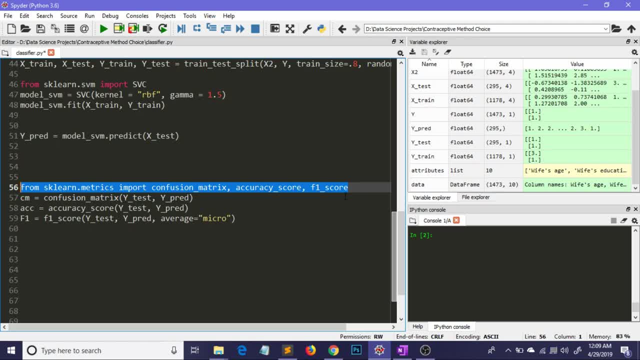 second one is accuracy score and the third one is f1 score. so let me just run this code so these classes are imported, and after that i'm going to declare an object of this class called confusion matrix and uh, to declare this i need to just write cm and then assignment operator and. 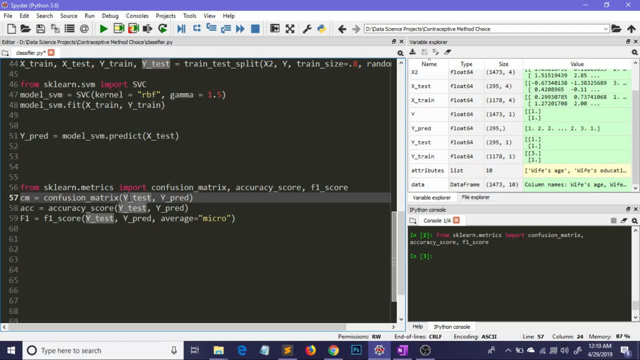 after that confusion matrix class and in the parenthesis, i have to pass the two arguments, which is the y test? well, y test represents the ground truths of our test set and the y pred represent the predictions on our test set. now, remember that i am using this confusion matrix in the test set, but generally, uh, we use the. 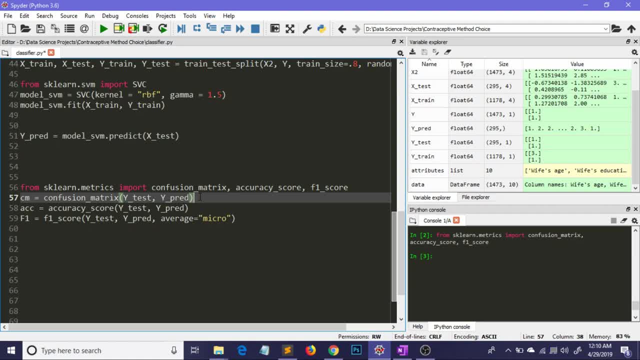 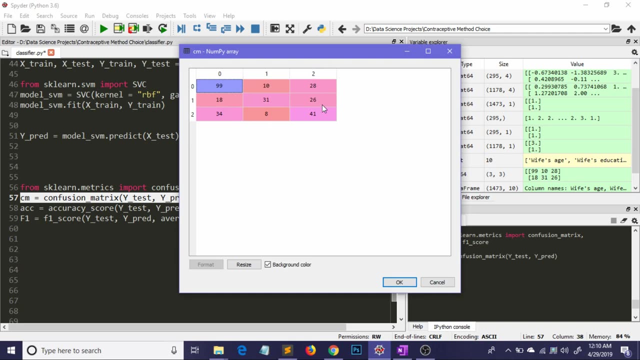 cost validation set to examine our model. okay, so keep that in the back of your mind. so i'm running this code and you can see that i have got this one here. so this is a matrix, this is a confusion matrix and in the conceptual part we just 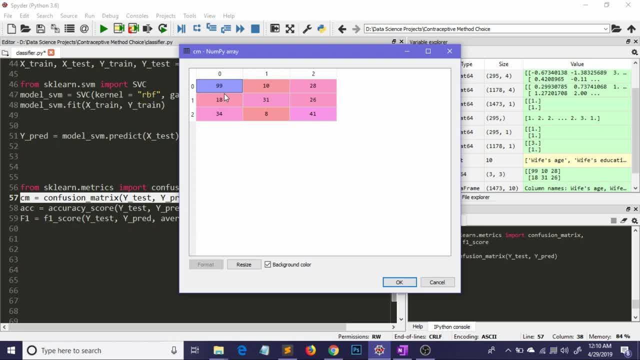 saw a smaller dimensional version that was a binary classification. we had just only four cells, but here, as we have three classes, we obviously going to have nine cells. so the diagonal cells represents the correct predictions and all the other cells represent the incorrect predictions and the we in case of binary classification, we may call uh this as true or the false positive and 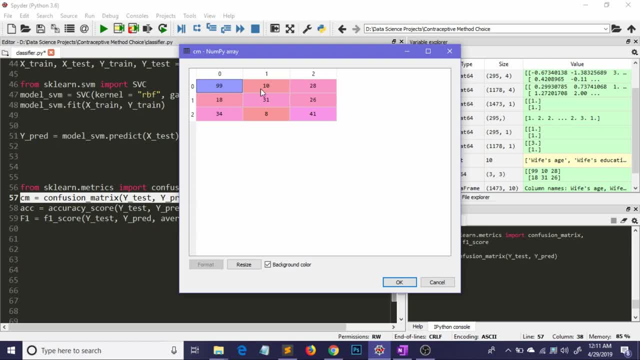 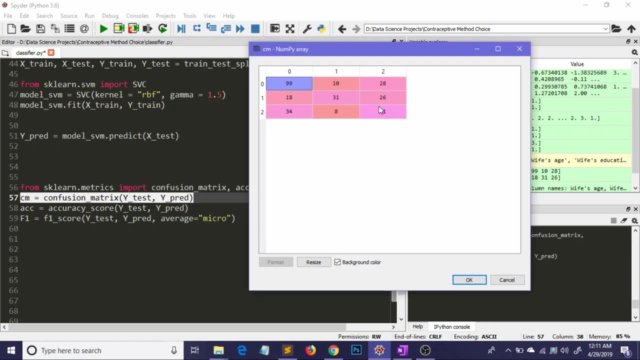 false negatives. okay, but here i'm going to call this that desquec. here we have four cases, so we don't usually call them as false positive and false negatives, right? so how to calculate the accuracy score here? well, to find the accuracy score here, we are going to just sum these things in the 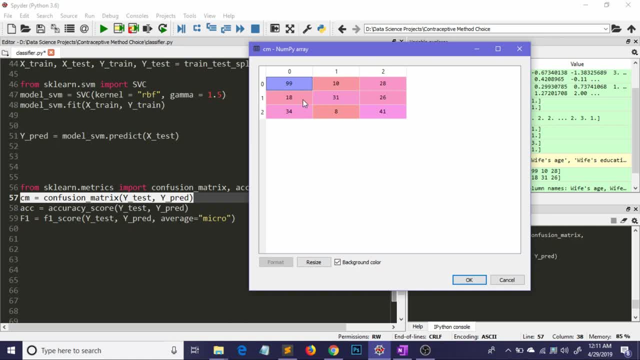 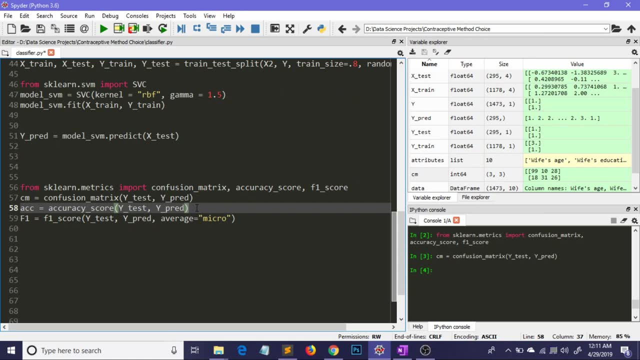 diagonal and we will be dividing by the total cells. okay, so that you can do it by the inbuilt class in the scikit-learn and by defining an object of this class, which is the accuracy object I have defined of the accuracy score class. and again, in the parentheses, I have to pass two arguments: the ground truth and the 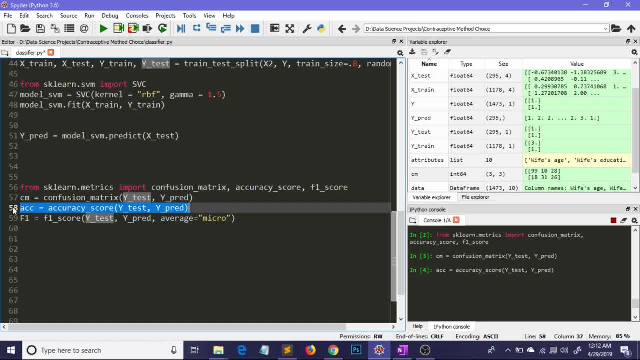 predictions. okay, so after I run this code I will have the accuracy here. so this is my accuracy now. remember it was try class classifications. so if we wouldn't have used any model, then we will get a acuity see of 0.33, ideally in the random guess case. but here I have implemented a model. 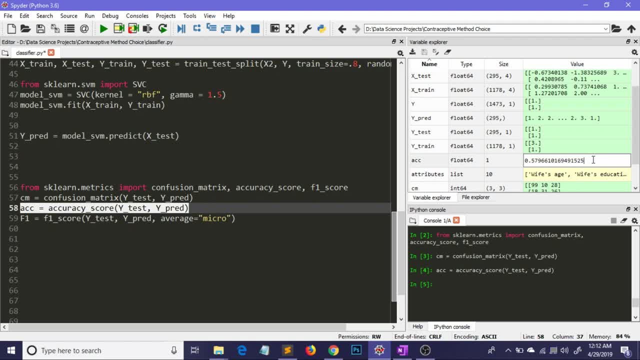 and I have got an accuracy of 0.57. now, remember, you can get actually accuracy far better than that, but this data set was a complex data set and so I couldn't manage to get more than this okay, so I will definitely link this data set to 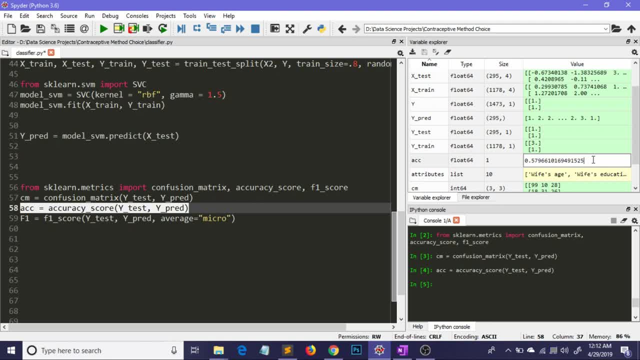 the description, and if any of you guys can come up with a better accuracy, then please let me know in the comments. so that was the accuracy score and finally, we are going to find the f? unsere score, which is also very easy to find in case of our scikit-learn. so just we need.